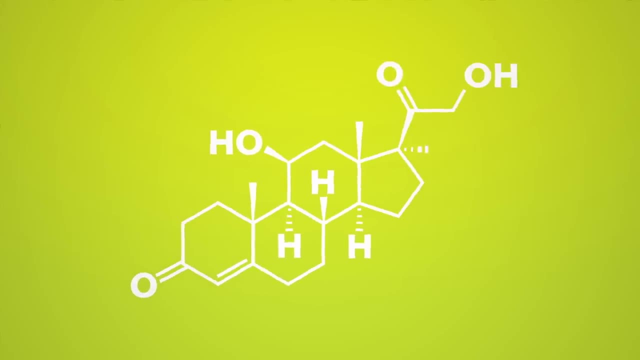 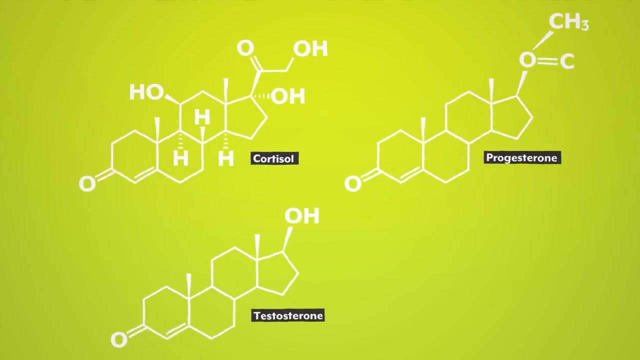 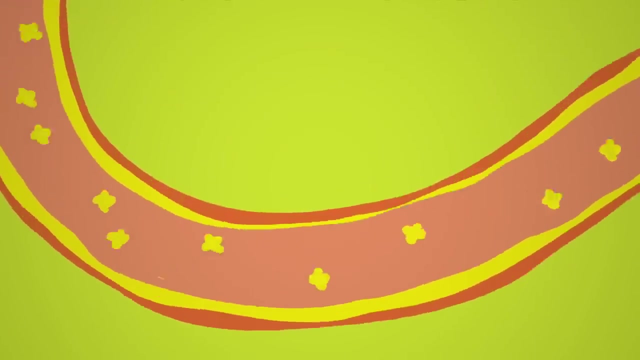 A molecule must contain this exact arrangement to be a steroid, though most also have side chains— additional atoms that can dramatically impact the molecule's function. Steroids get their name from the fatty molecule, cholesterol. In fact, our bodies make steroids out of cholesterol. 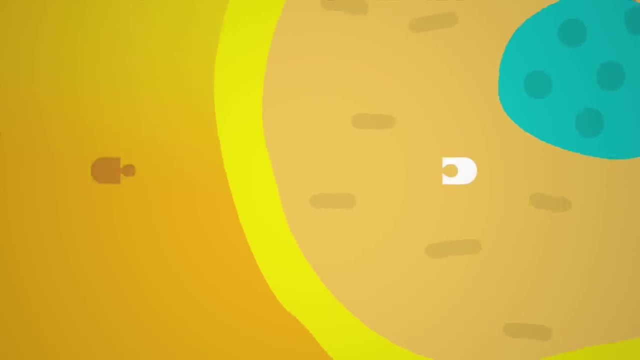 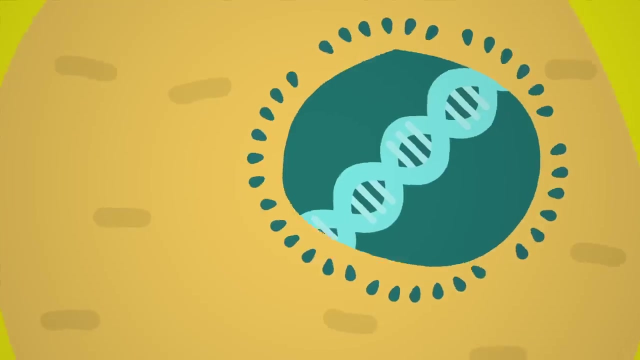 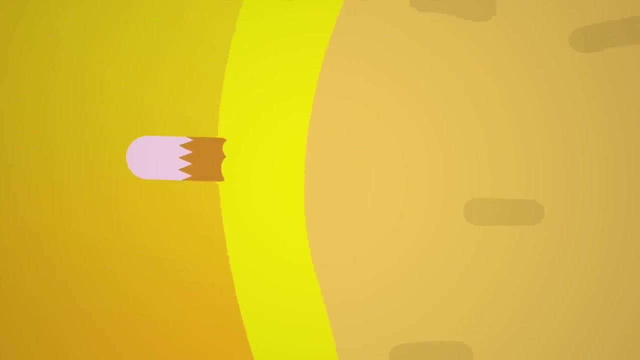 That fatty cholesterol base means that steroids are able to cross fatty cell membranes and enter cells Within the cell they contain that directly influence gene expression and protein synthesis. This is different from many other types of signaling molecules which can't cross the cell membrane. 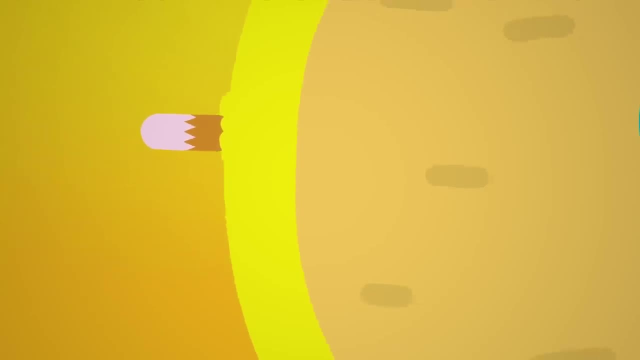 and have to create their effects from outside the cell through more complicated pathways. So steroids can create their effects faster than those other molecules. Back to the steroids in anti-inflammatory medications. All of these are based on a naturally occurring steroid called cortisol. Cortisol is the body's primary stress signal. 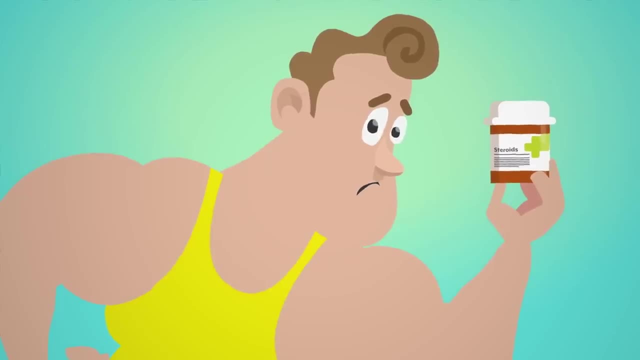 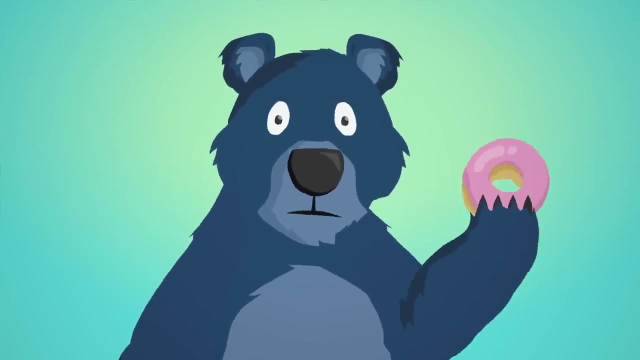 and it has a huge range of functions. When we experience a stressor- anything from a fight with a friend to spotting a bear, to an infection or low blood sugar- the brain reacts by sending a signal from the hypothalamus to the pituitary gland. The pituitary gland then sends a signal to the adrenal glands. The adrenal glands produce cortisol and release some constantly, But when they receive this signal from the pituitary gland, they release a burst of cortisol which spurs the body to generate more glucose for energy. decrease functions not immediately related to survival, like digestion, and can activate a fight, flight or freeze response. This is helpful in the short term, but can cause undesirable side effects like insomnia and lowered mood if they last too long. Cortisol also interacts with the immune system. 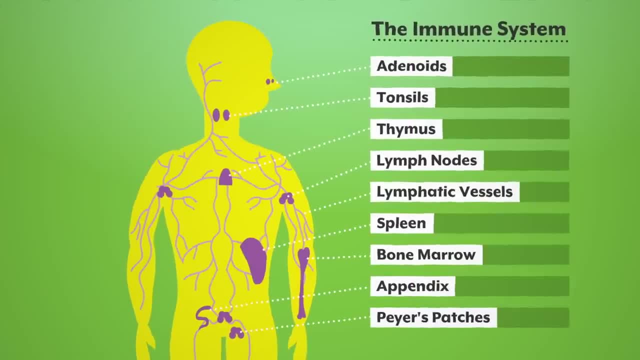 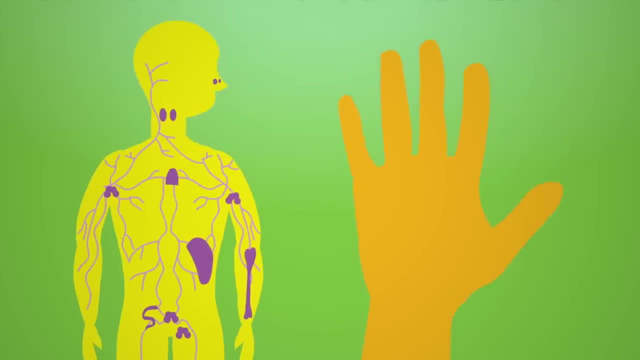 in common. In complex ways, depending on the situation, it can increase or decrease certain immune functions. In the process of fighting infection, the immune system often creates inflammation. Cortisol suppresses the immune system's ability to produce inflammation, which again can be useful in the short term. 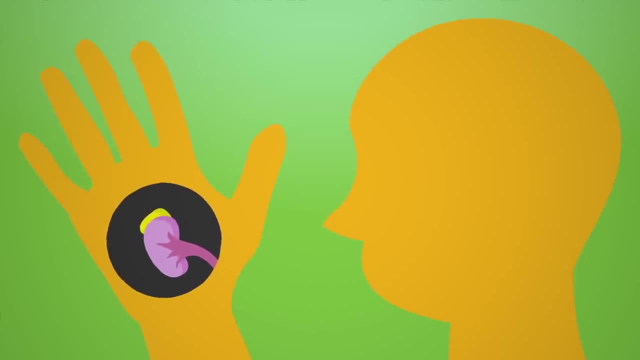 But too much cortisol can have negative impacts like reducing the immune system's ability to regenerate bone marrow and lymph nodes To prevent levels from staying high for too long. cortisol suppresses the signal that causes the adrenal glands to release more cortisol. Medicinal corticosteroids channel cortisol's effects on the immune system. 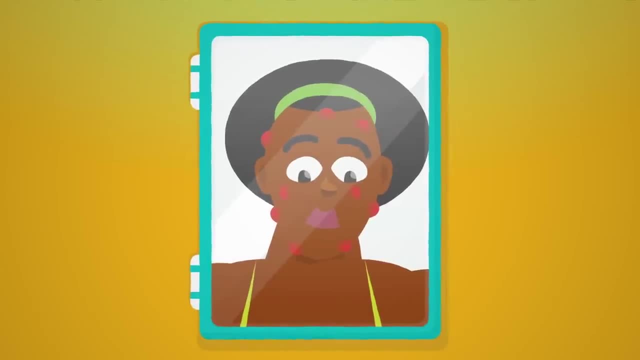 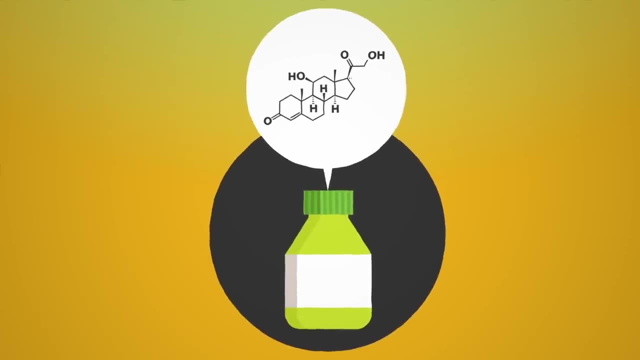 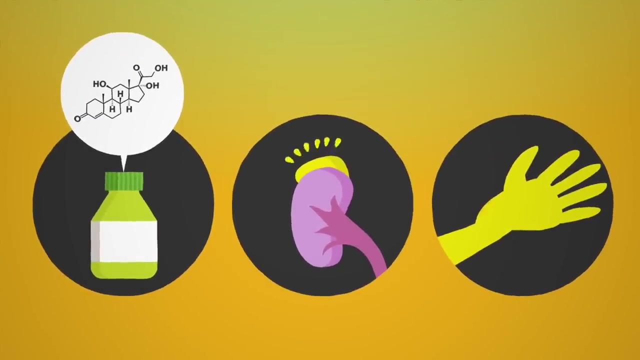 to fight allergic reactions, rashes and asthma. All these things are forms of inflammation. There are many synthetic steroids that share the same basic mechanism: They enhance the body's cortisol supply, which in turn shuts down the hyperactive immune responses that cause inflammation.